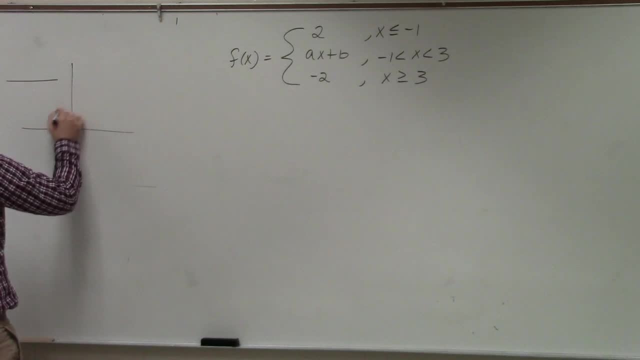 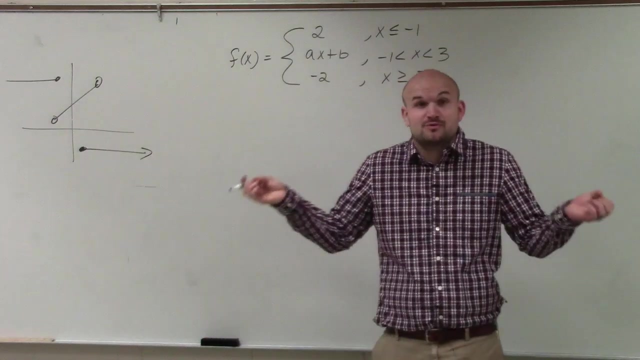 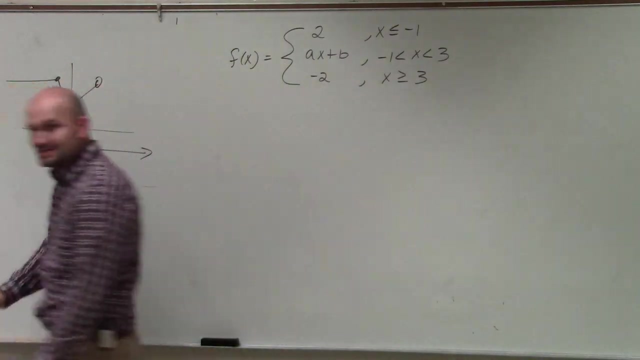 graph looks something like this: You have two, then you have this line and then you have like negative two, right? It looks something like that. roughly I'm not even I didn't even check the numbers, but it looks something like that. So there's two points where it could be, where it could be breaks. So we need to find the values of A and B. where it's going to connect right, So it's going to be continuous. That's what the question is asking. So, again, first thing we need to do is find the values of A and B. 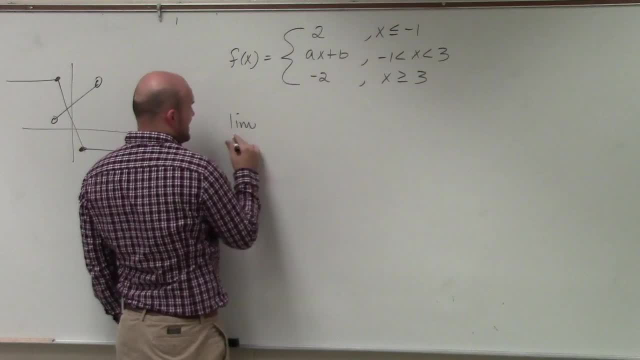 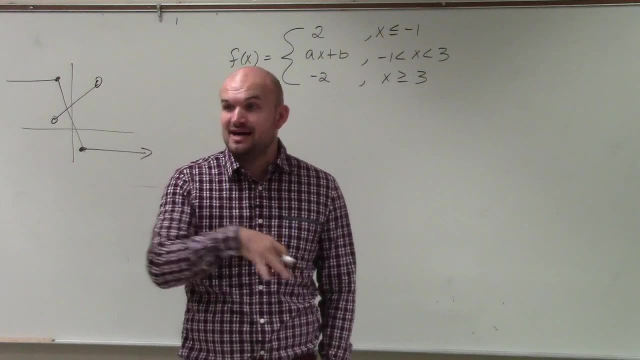 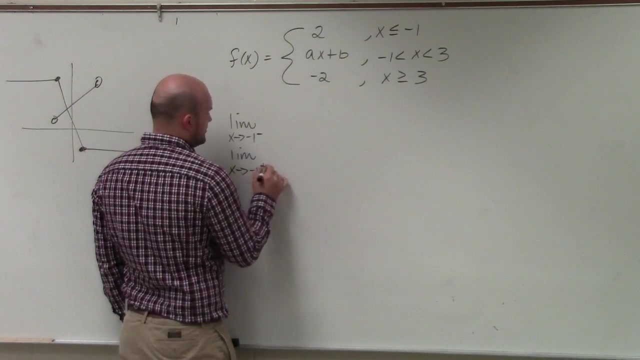 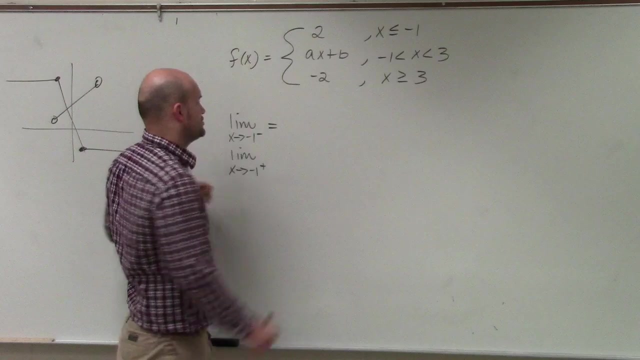 Second thing we need to do is evaluate, for the limit at x equals negative one. We need to make sure that limit exists. so, therefore, to do that, we need to check the limit from the left-hand side and from the right-hand side. So let's do limit from the left and the limit as x approaches negative one from the right- Well, from the left- is going to be the values that are less than negative, one which is just two. The limit of any constant is obviously just going to be two there. 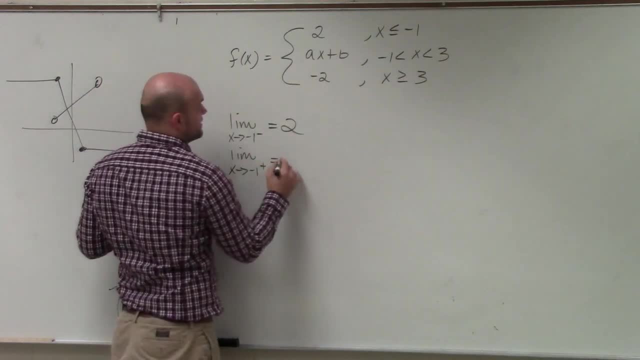 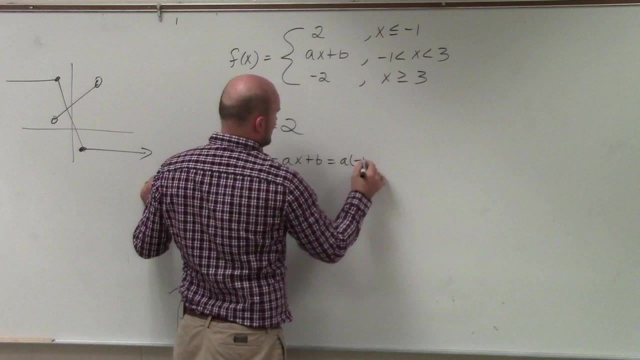 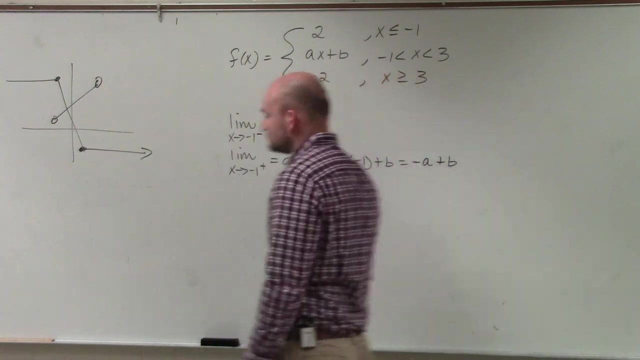 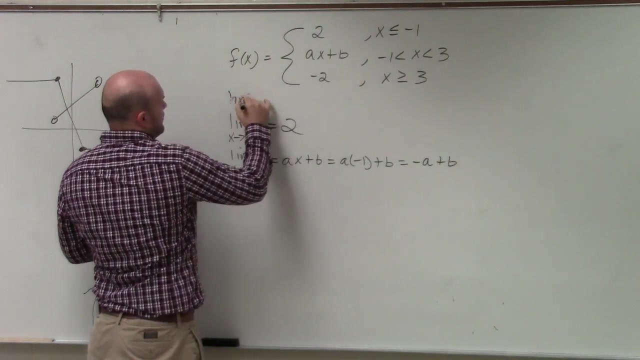 the right, we have ax plus b, So that's going to be ax plus b. Well, if we evaluate here negative 1, that's going to be a times negative 1 plus b, which equals negative a plus b. Now again for our limit. let me actually write this one For our limit as x to approach. 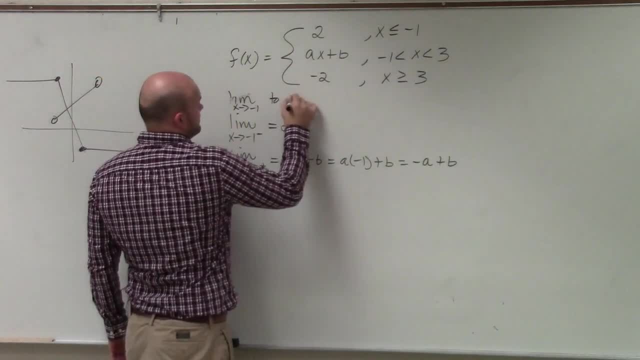 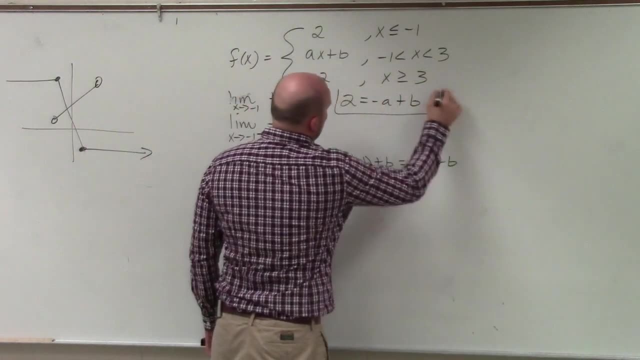 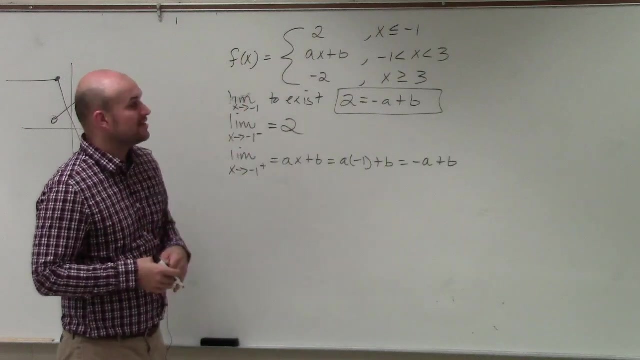 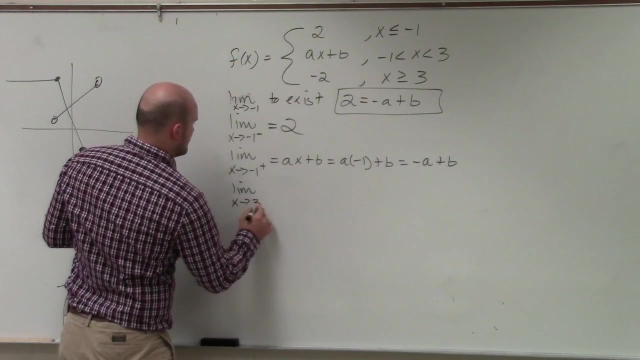 negative 1. to exist, 2 has to equal negative a plus b. We're just going to keep that. We're going to store that. Now let's look at the next break-even point At 3, the limit as x approaches 3 from the left. So 3 from the left is going to be the left. 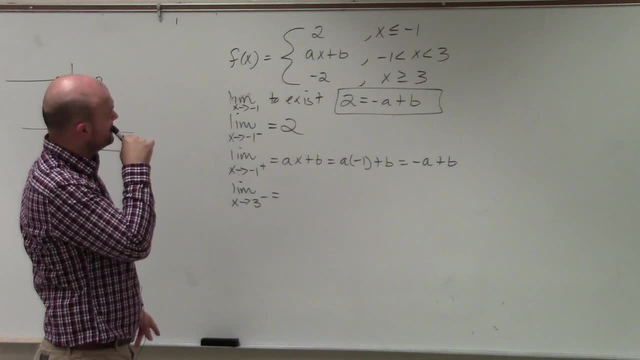 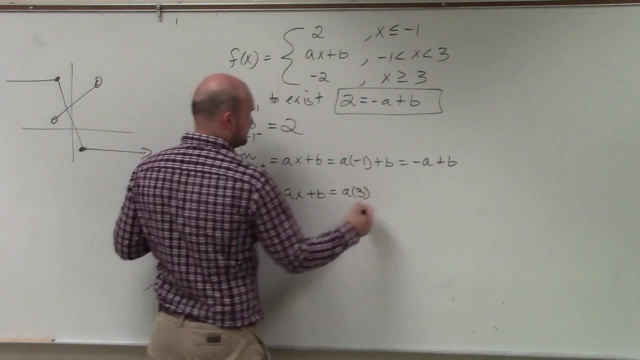 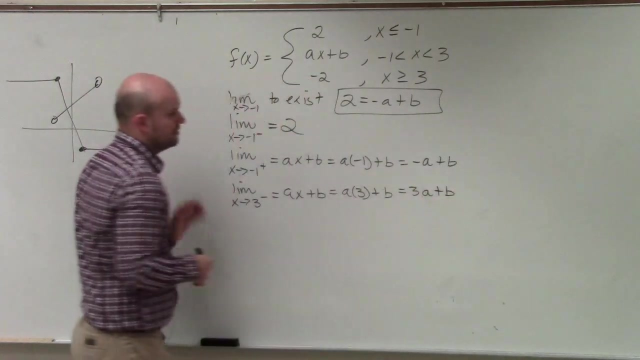 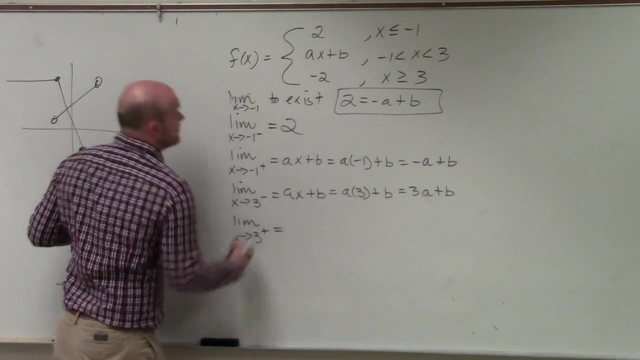 Is that 3?? Is going to be ax plus b. Evaluate for the limit 3.. 3a plus b. Does everybody follow Limit as x approaches 3 from the right is just negative. 2. Again for the limit as. 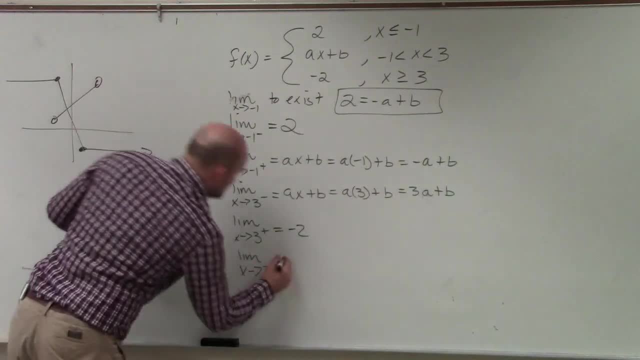 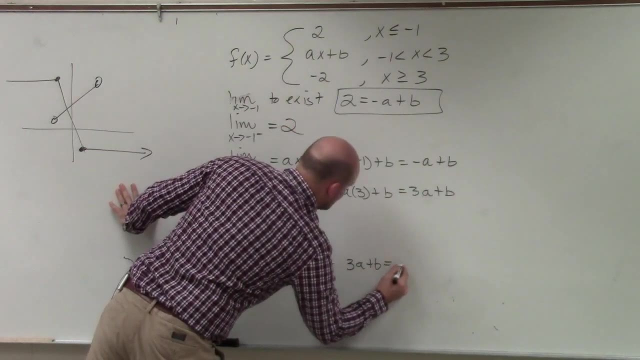 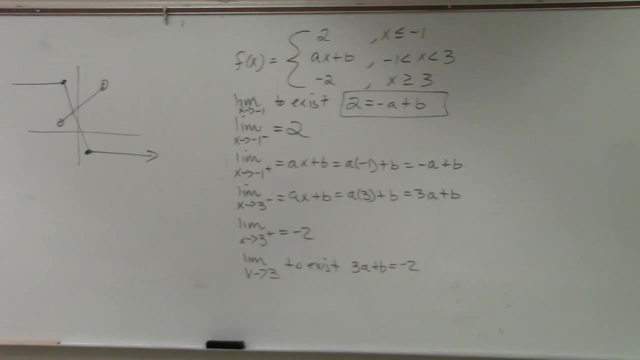 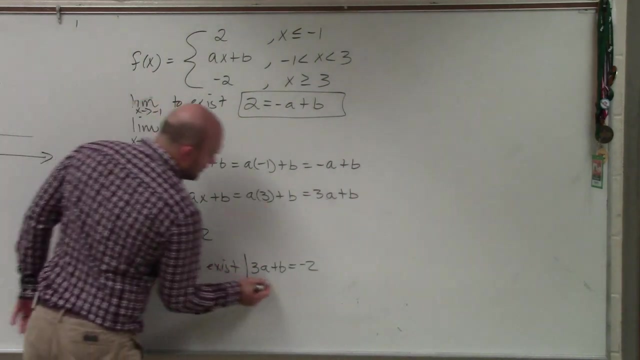 x approaches 3 from the left. 3a plus b has to equal negative 2.. So now we have two equations where we know that the limit needs to exist. So for this to be continuous, limit at 3 needs to exist and the limit at 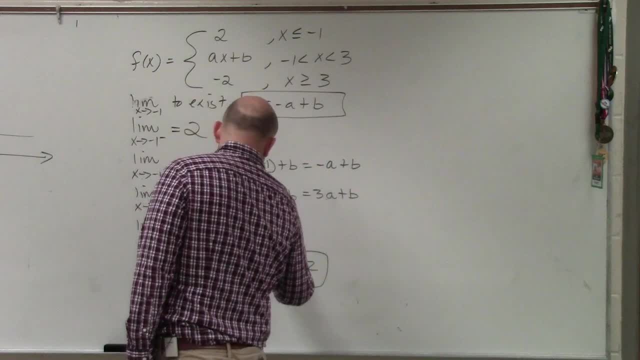 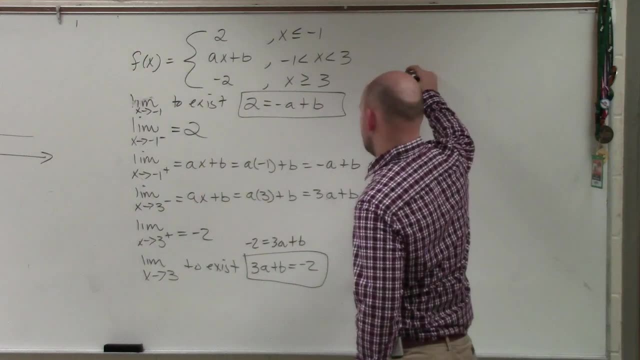 2 needs to exist. I'm just going to rewrite this. I'm going to rewrite this as negative: 2 equals 3a plus b, If that's OK with you guys, just using the reflexive property. So, therefore, what I have is system of equations. 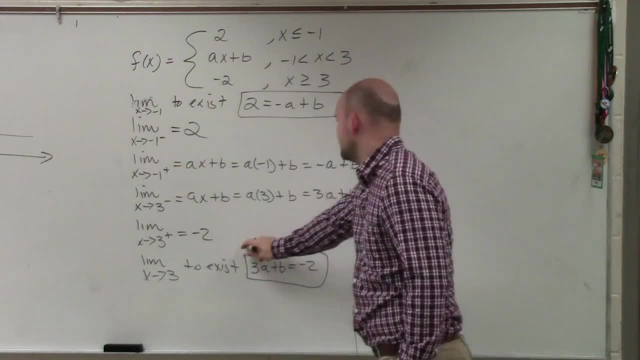 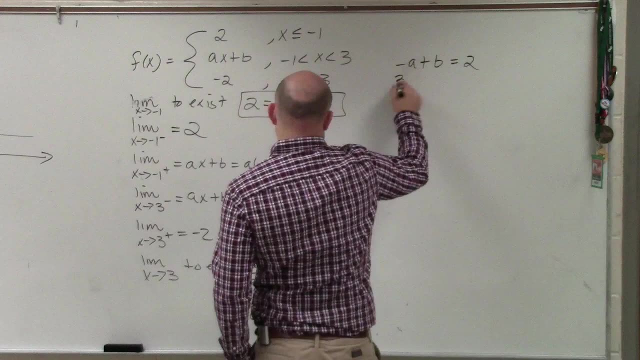 I have two. Actually, let's rewrite it. Actually, I'm going to leave that like that. I'm going to rewrite this one, So I'll have negative a plus b equals 2.. And I have 3a plus b equals negative 2.. 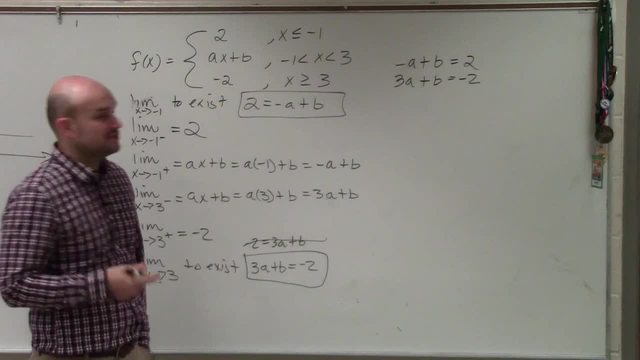 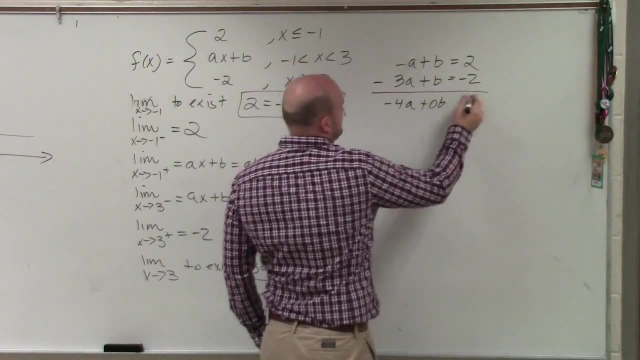 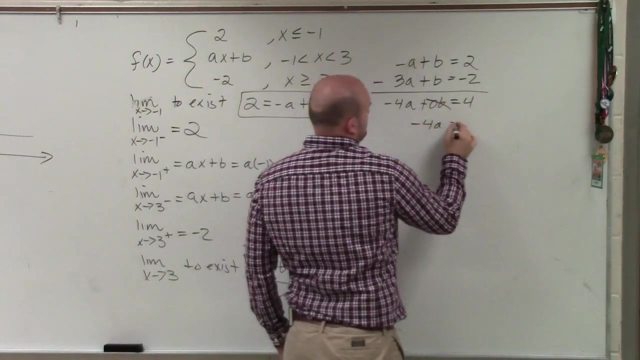 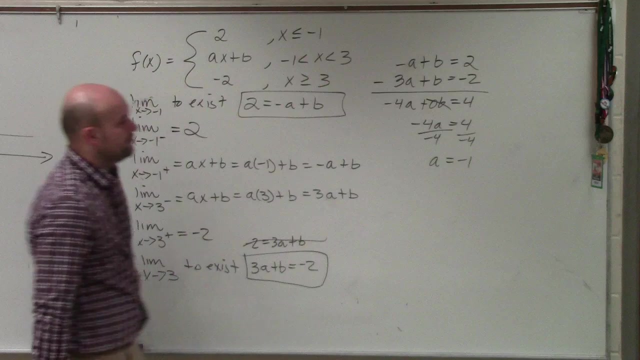 And then to solve the system of equations, I could use substitution, or I could also use elimination, Or I could just subtract them. So therefore I figured out: a is equal to negative. 1. Where 3a plus b, 3a plus b. 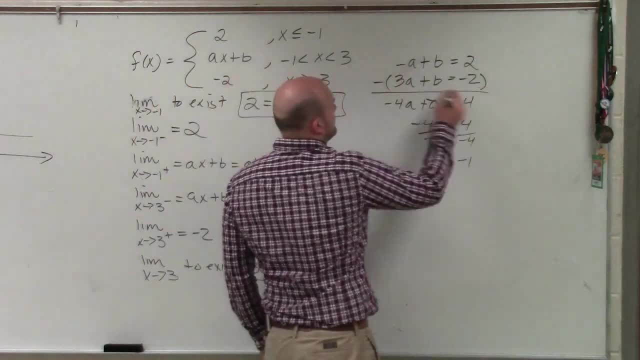 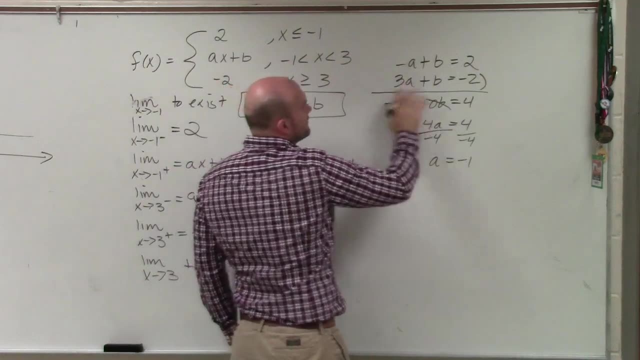 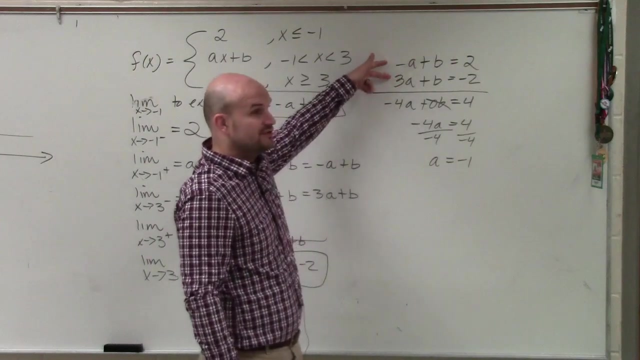 Yeah, I'm subtracting each of these rows Here. That's the two equations, right? Do you see these two equations? Do you agree with me? Do you have these two equations? Okay, So these are the two equations in my system. 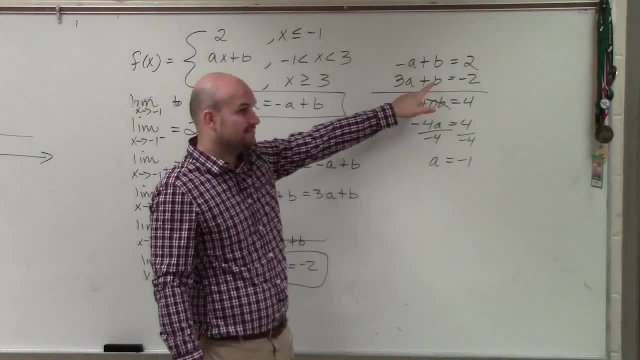 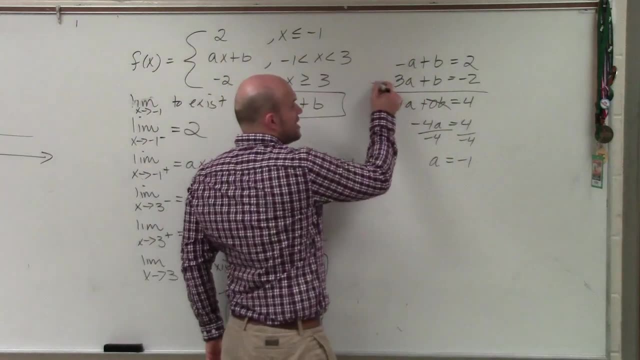 I need to eliminate B. Well, I can't add them right, because that's going to give me 2A and 2B, So I have to subtract the equations. So I'm going to subtract the bottom equation from the top equation. 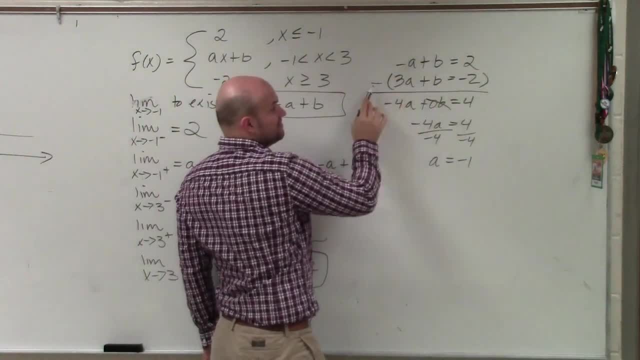 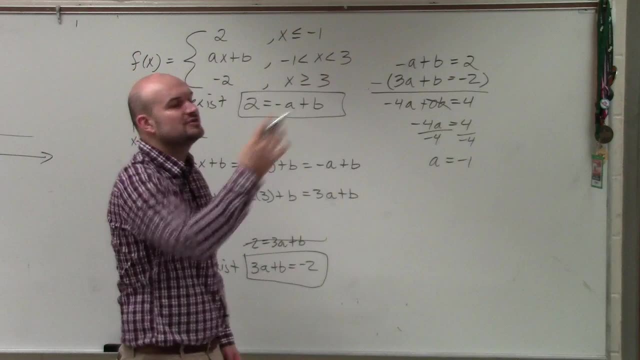 So it's negative A minus 3A, It's negative 4A. B minus B is 0B, 2 minus a. negative 2 is 4.. Try your way another. Do substitution your way Right, Substitute and solve for A or B.